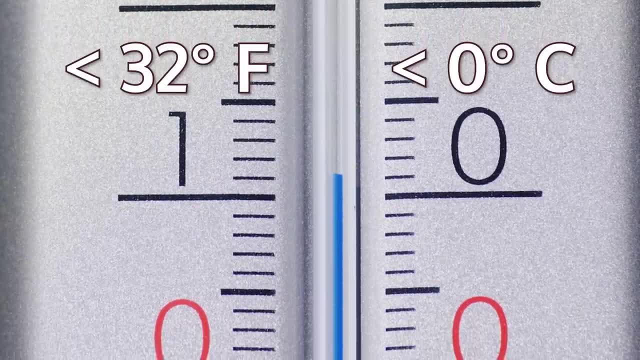 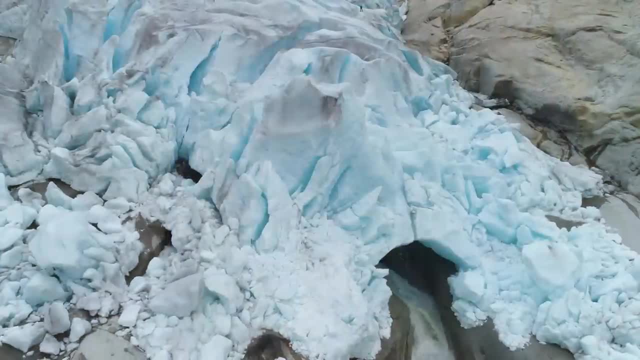 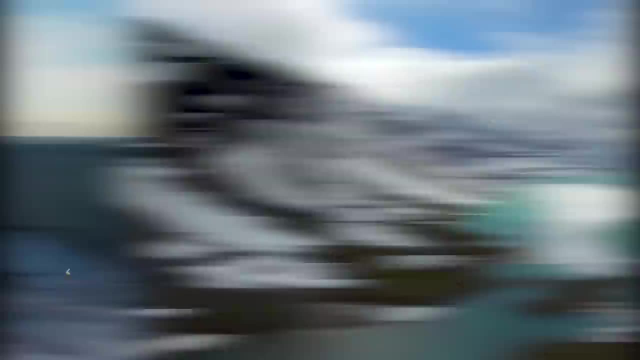 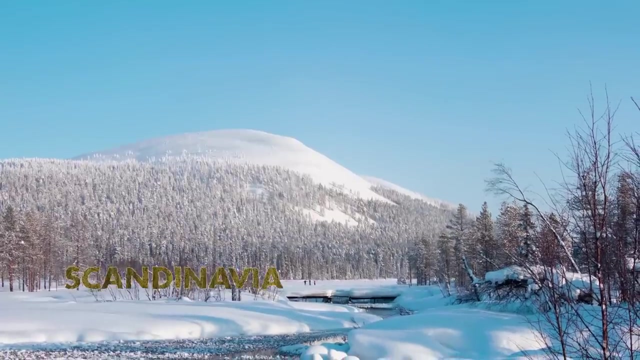 In fact, it never gets above freezing, But for a short time the temperatures in the Arctic or north pole may rise above freezing and the ice can melt. Just south of the Arctic Circle there are sub-Arctic areas. These include Greenland, Alaska, northern Canada and the northern areas of Scandinavia and Siberia. 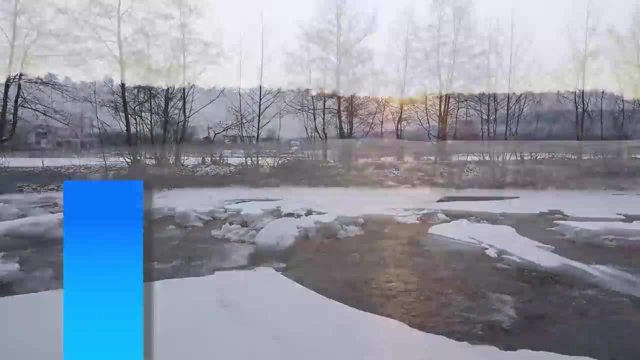 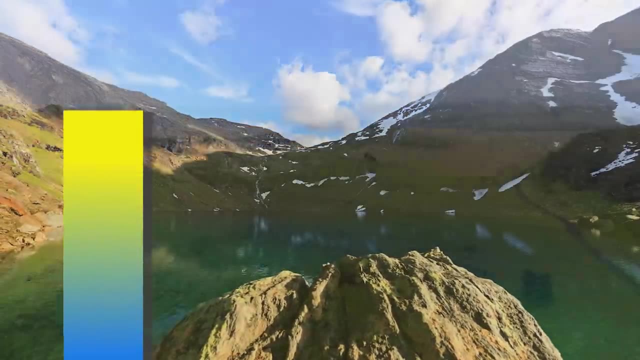 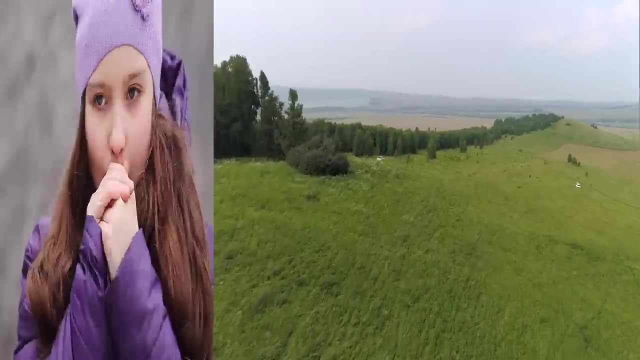 In winter, the temperature is below zero and the rivers and lakes are frozen, But in summer, when temperatures rise above freezing, the ice melts and plants that grow on the tundra can support some animal life, If you don't like being cold or living where there isn't sunlight for long periods of time. 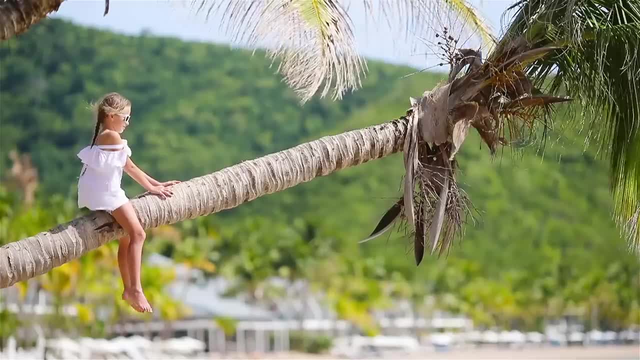 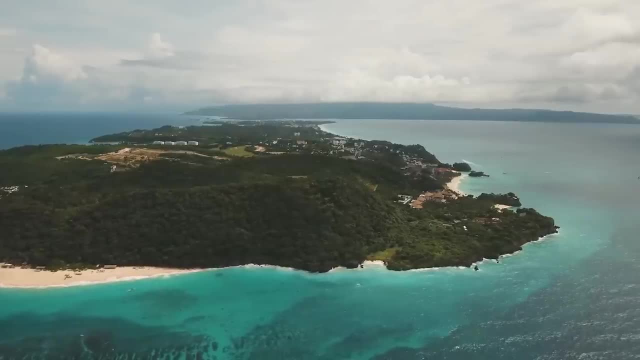 then the Arctic is not the place for you. Instead, you may prefer a tropical climate. A tropical climate is a climate in a tropical region. Tropical climates are just north and south of the equator. Tropical climates are forests that areỉ near the equator. 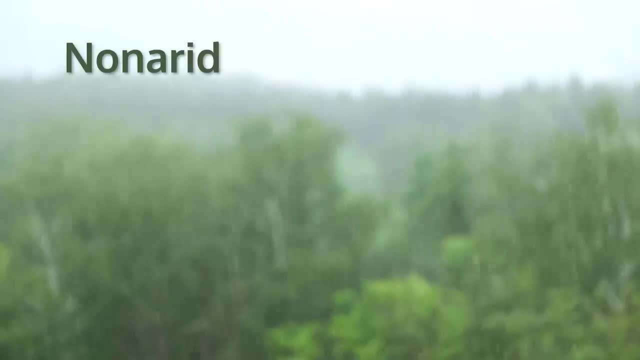 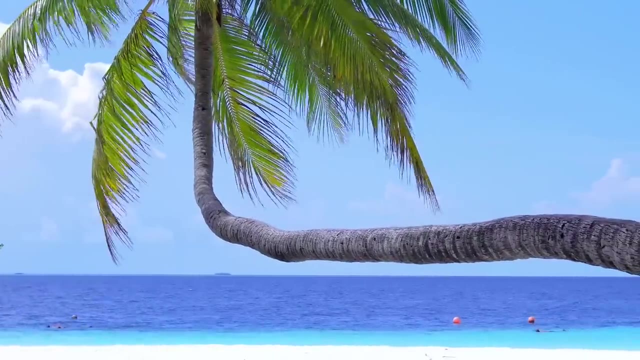 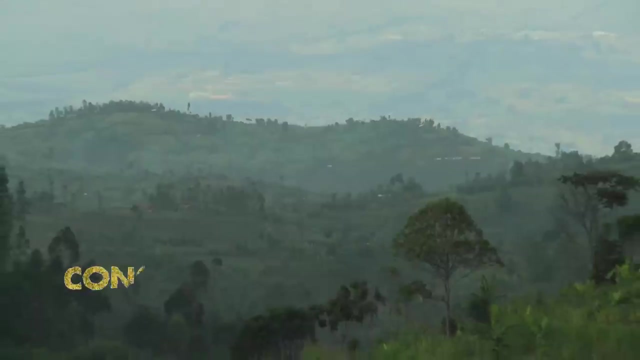 Non-arid climates are non-arid climates. Non-arid means they get a lot of rain, especially in the summertime. The temperatures are very warm in tropical climates. Even in winter, where there is less rain, it's still warm. The Congo in West Africa and the Amazon in Brazil are both examples of tropical climates. 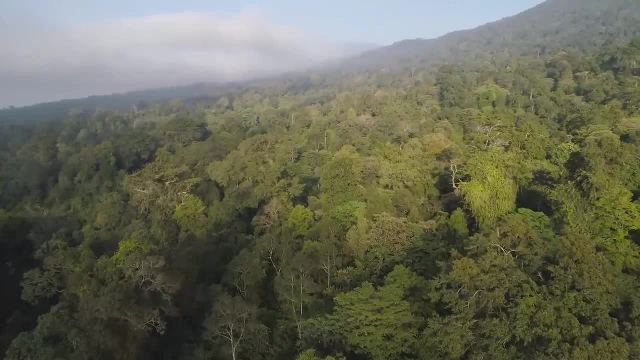 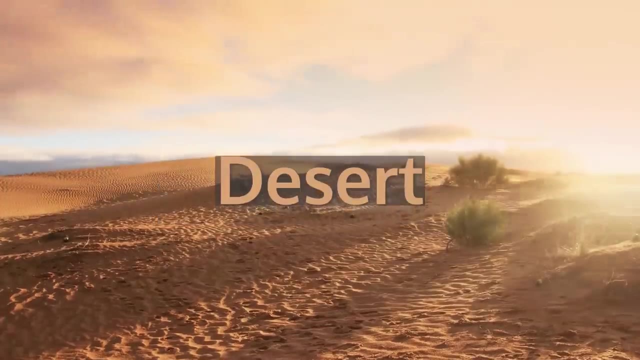 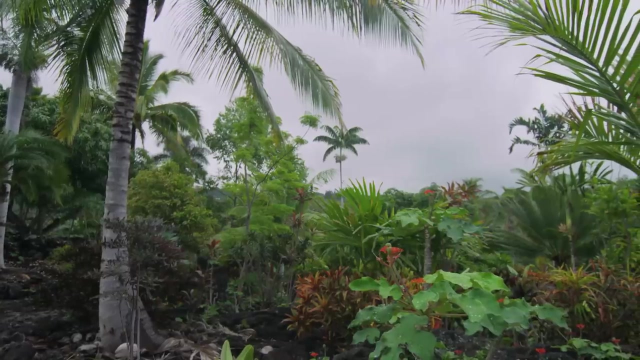 as well as some rainforests. in Malaysia and Indonesia There are two types of tropical climates: equatorial and desert. Equatorial climates run along the equator. The temperatures are warm in these locations year-round. Rain falls all year in these areas as well. 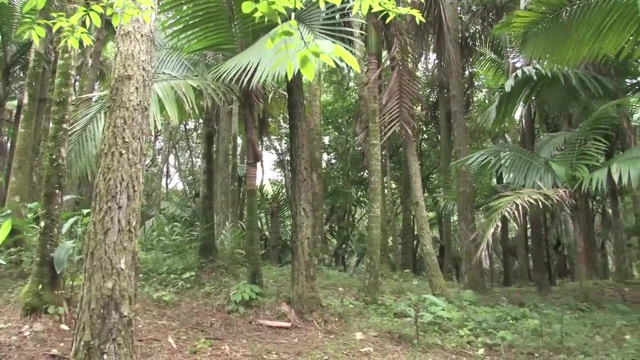 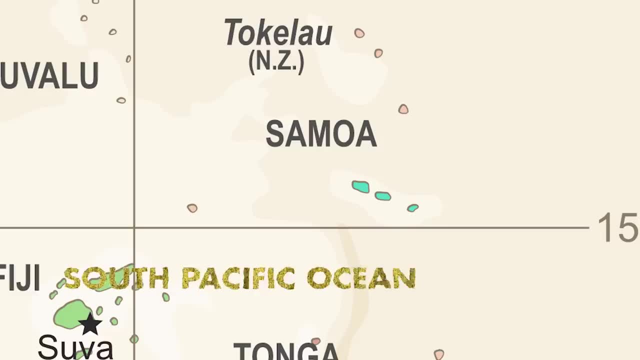 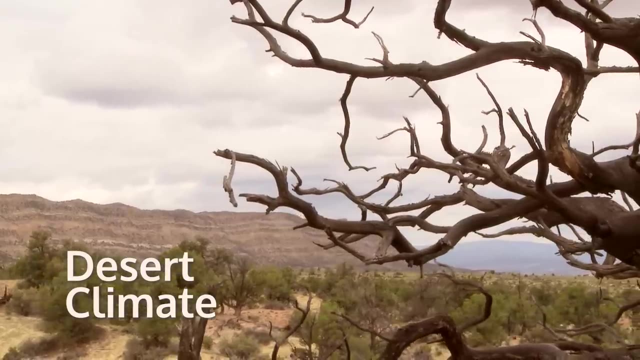 During the summer it gets very hot and humid, and when it rains it usually occurs with thunderstorms. Fiji, Samoa and Tonga are examples of equatorial climates. Desert climates are very dry and hot. They get very little or no rain at all. 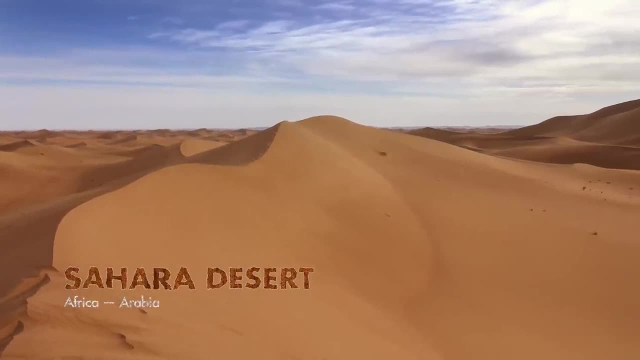 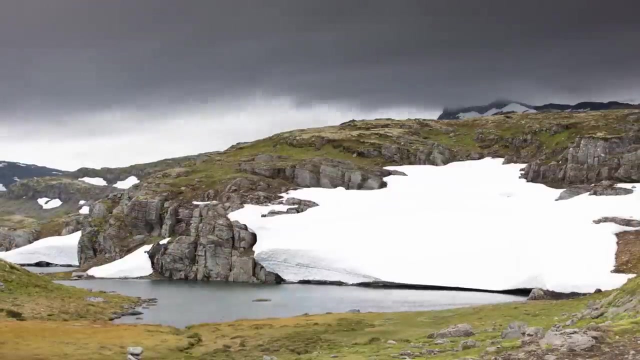 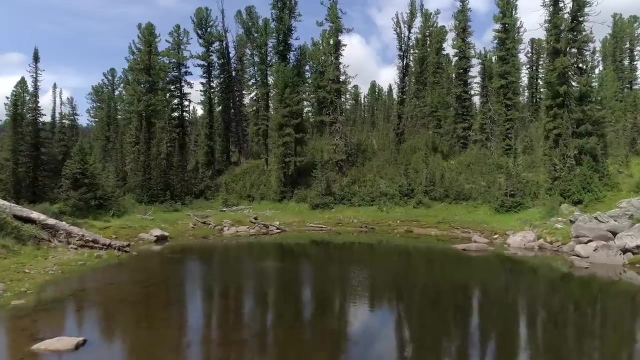 Desert climates are found in North Africa, such as the Sahara Desert, in Arabia and in parts of Australia. If you don't like the idea of living in a very cold Arctic climate or a very hot tropical climate, then perhaps you need something in the middle. 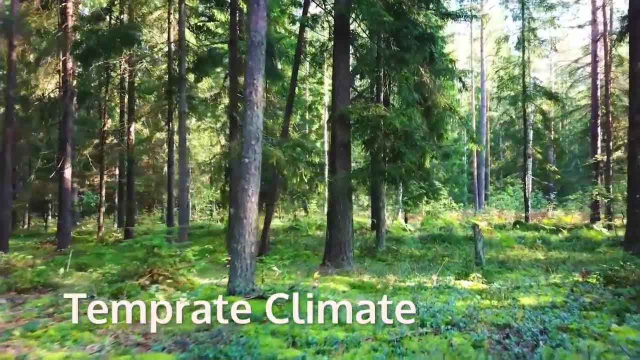 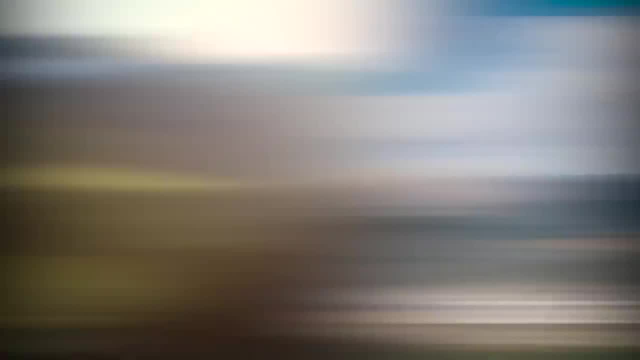 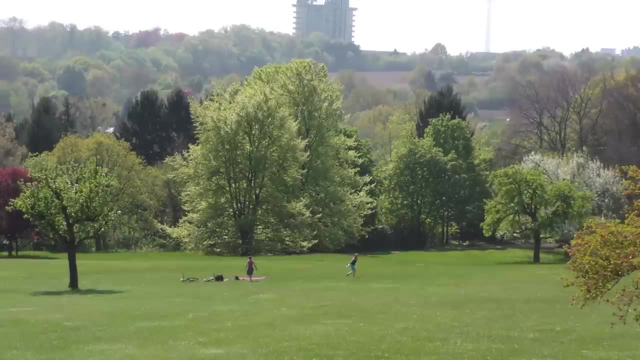 In a temperate climate, it doesn't get very hot or very cold. Instead, the temperature usually stays about the same. Most of Canada, Europe, Central Asia and southern parts of Australia and South America are all places that have temperate climates. 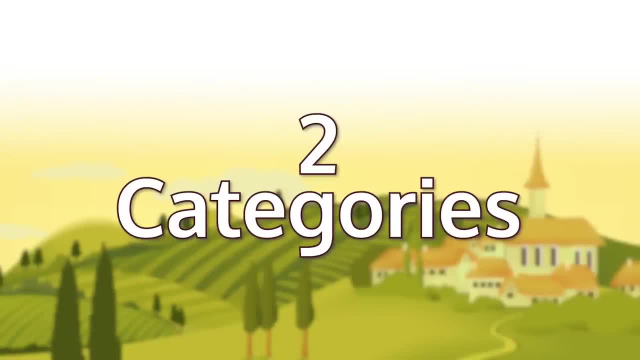 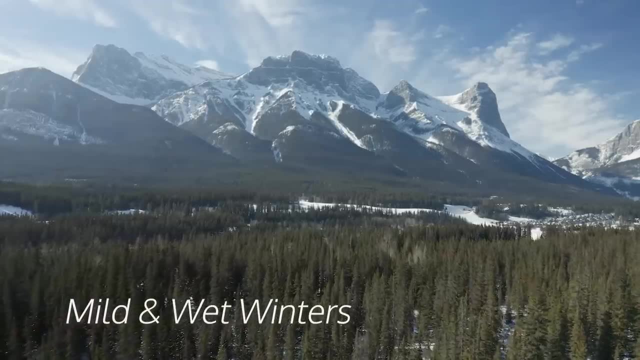 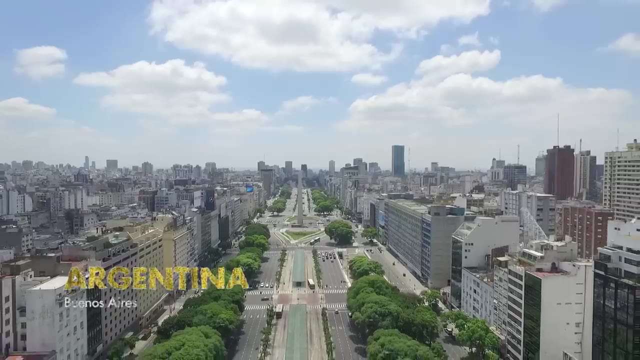 There are two categories of temperate climates: Warm and cool. In warm climates, the winters are usually mild and wet and the summers are hot and dry. Some areas of Chile and Argentina, as well as Southern California, are examples of warm climates. The Mediterranean, where Greece and parts of France, Italy and Spain are located, are also warm climates. In cool climates, the winters are cold and the summers are warm. The winter months have snow and freezing temperatures for short periods of time. 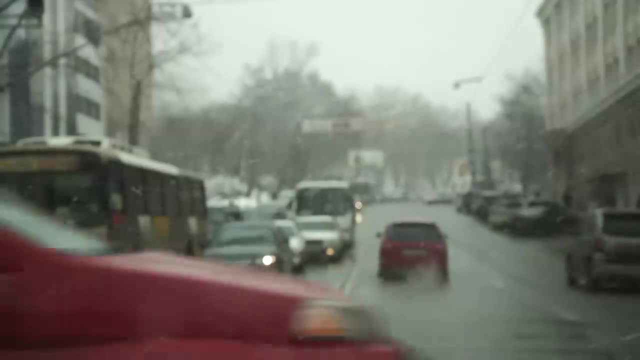 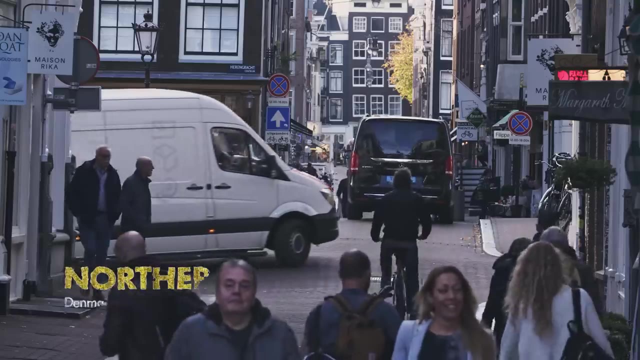 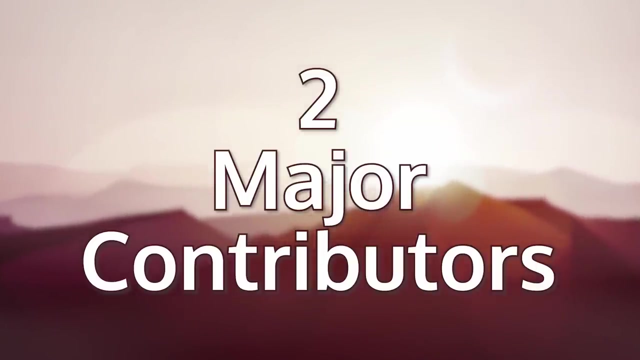 and there is less rain in the summer than there is in winter. Examples of cool climates include the British Isles, Northern Europe and New Zealand. Two major contributors to an area's climate are how close an area is to the ocean and how high above sea level it is. 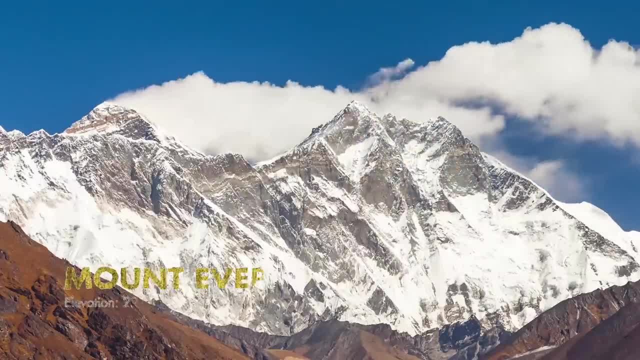 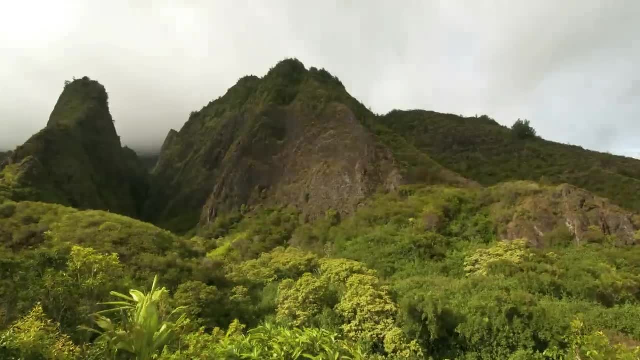 There is much room for change in the climate. The higher the elevation, the colder the climate, and the lower the elevation, the warmer the climate. For example, if you were to climb a mountain in a warm area, the higher you get. 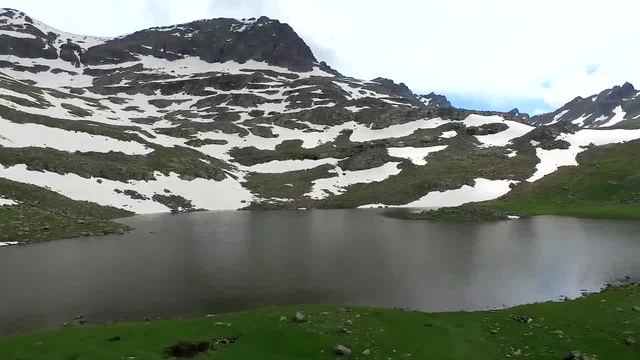 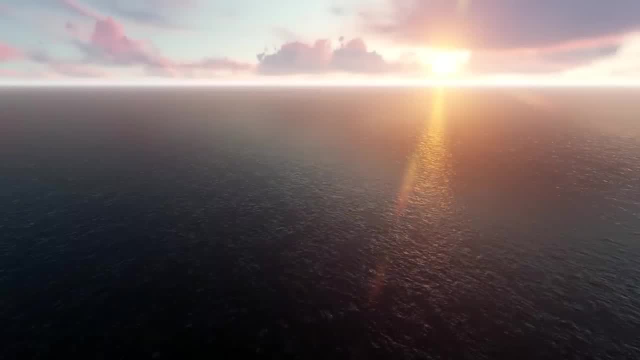 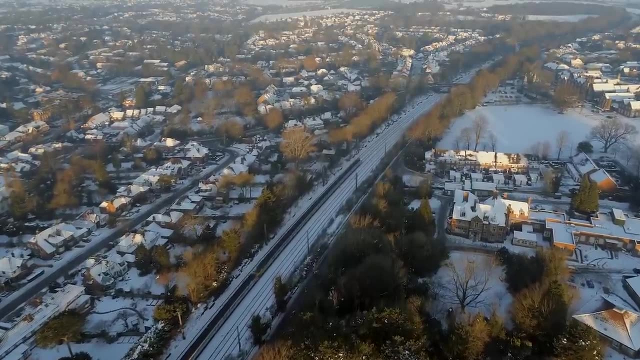 the cooler it becomes and the climate is no longer a warm one. Oceans and seas affect climates too, by absorbing the heat from the sun. That's why it's warmer nearer the coast and cooler further away. Hot or cold winds also affect the climate. 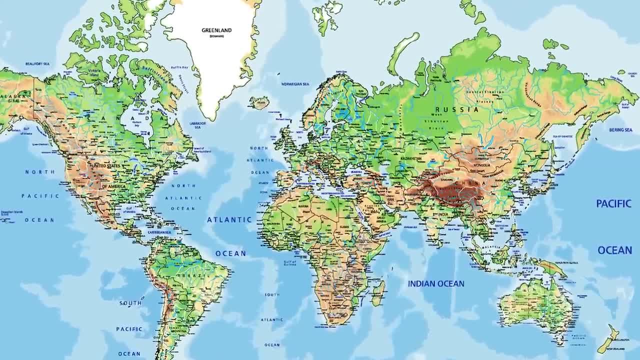 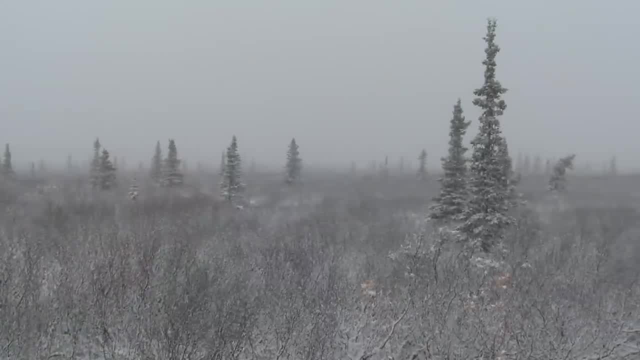 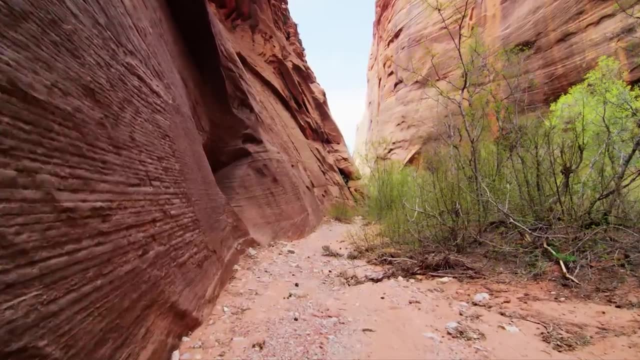 Climates can vary drastically inside a single country. The United States is one, for example. Hawaii is a tropical climate, Alaska is part of the sub-Arctic climate And within the other 48 states there are desert areas, rainy areas and dry climates. The warmest areas.